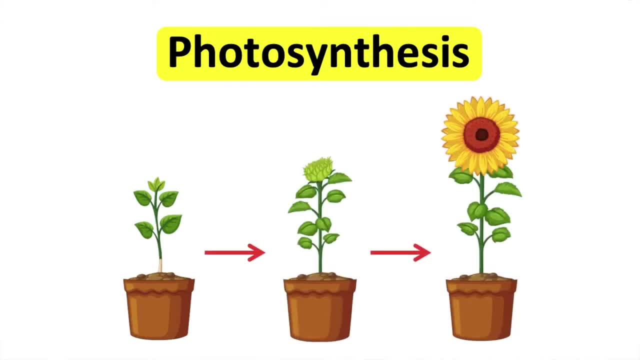 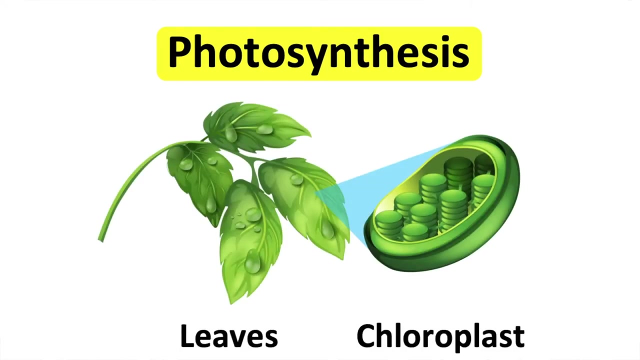 So plants need food to respire, to grow and to reproduce. Plants are producers. This means that they are able to make their own food. They do this by the process of photosynthesis. Photosynthesis takes place in the leaves of plants, specifically in the chloroplasts of 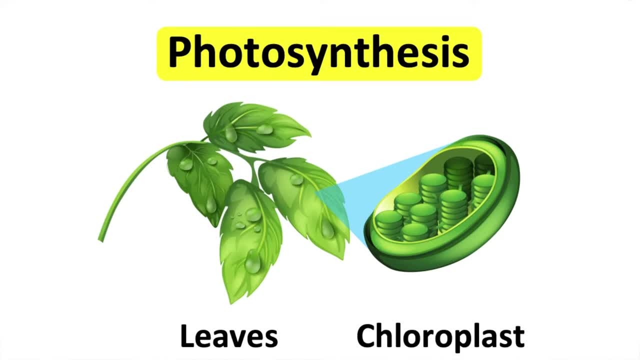 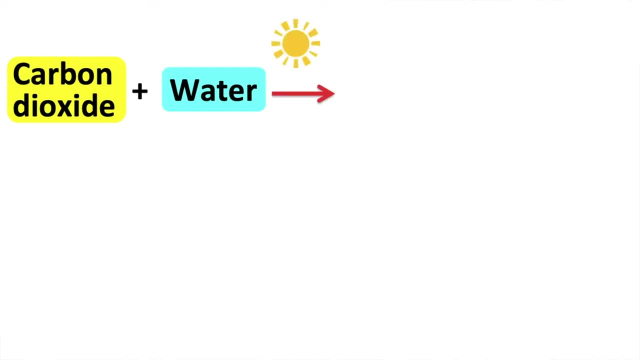 leaves containing chlorophyll. The equation for photosynthesis is the following: The formula for photosynthesis is carbon dioxide from the air, water and light energy, usually from sunlight. This reaction produces oxygen and glucose. The formula for carbon dioxide is CO2.. The formula for water is H2O. The formula for oxygen is O2.. The formula for glucose. 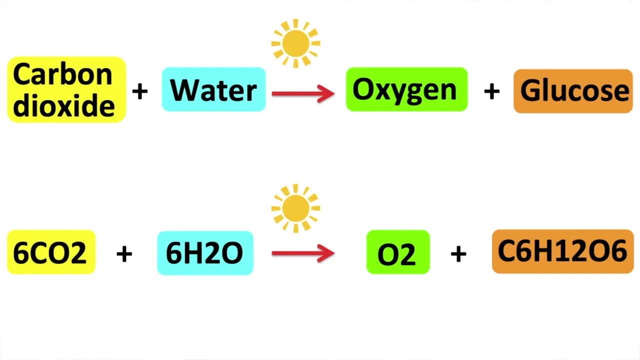 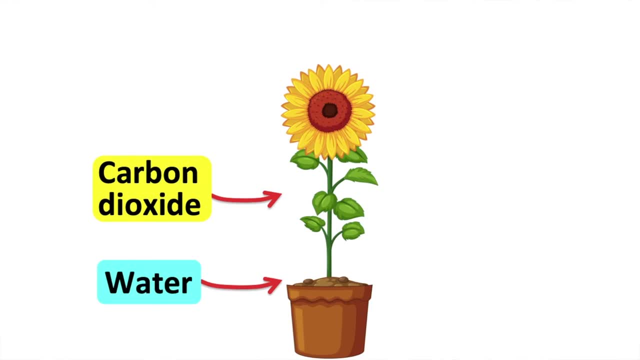 is C6.. Firstly, carbon dioxide and water enter the leaf. Carbon dioxide enters through the stomata of the leaf via diffusion. Water is absorbed by the roots from the soil. This water is then transported to the leaves by the xylem vessels. Sunlight provides the energy for. 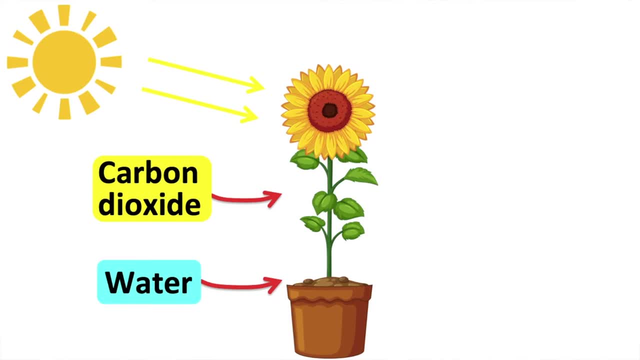 the process to take place. Hydrophil in plants can absorb the light energy. The products are oxygen and glucose. Oxygen is released back into the air and it's released through the stomata of the leaf. Glucose is a source of energy for the plant. Glucose is transported around the plant by 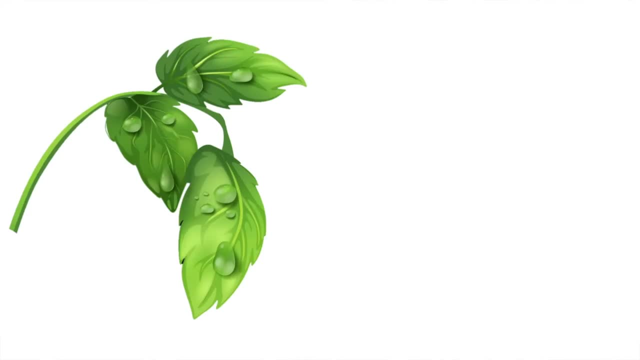 the phloem vessels. Photosynthesis is standardized. Leaves are adapted for photosynthesis by both heat and air. The photosynthesis process is photosynthesis in a few different ways. Firstly, leaves are big and they have a large surface area. This allows more sunlight to be absorbed. Secondly, leaves are green due to the chlorophyll. 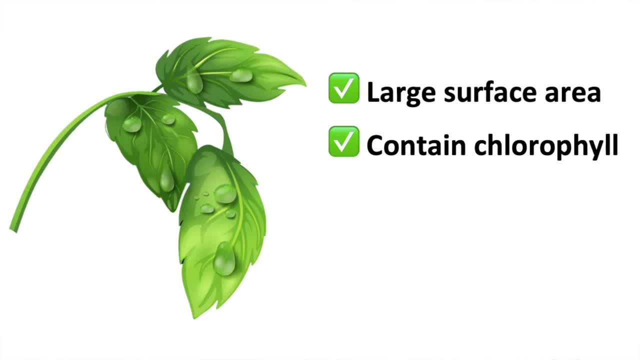 in the chloroplasts. This helps them to absorb sunlight. Thirdly, leaves are thin, which allows the diffusion of gases in and out of the leaf. Fourthly, the leaves have vascular tissues. Tubes that carry food from the leaves to the rest of the plant are known as phloem.